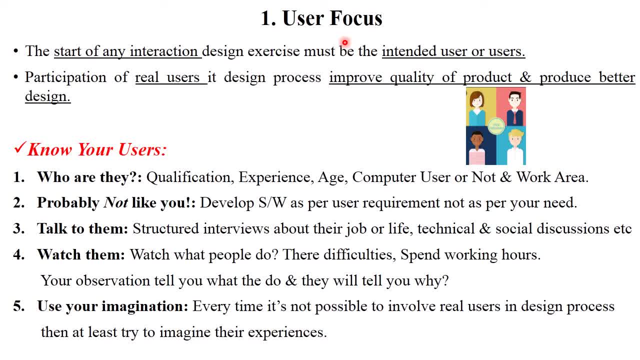 There are multiple users- single users. role of each and every user in interaction design. There are multiple users, single users. role of each and every user in interaction design is one of the most key part, or the most important part, of the software designing life cycle. 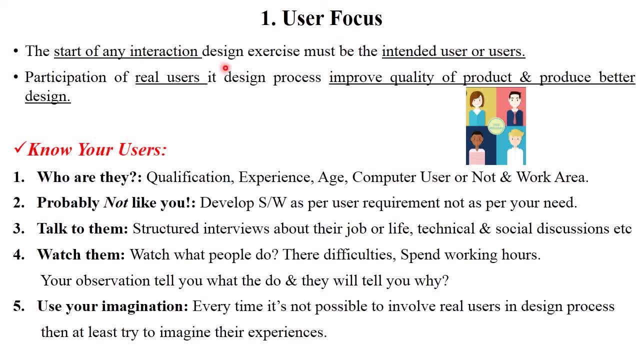 We all know that. So to start any interaction design exercise must be the intended users. So to start any interaction design exercise must be the intended users. Participation of real users in design process. it improve the quality of product. but its not enough to make data at a service level, not easily address standing case from the community. 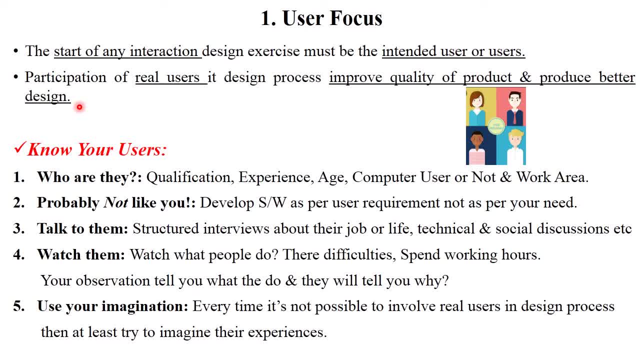 quality of product and produce the better design. if you should make a particular software as per the user requirement or customer requirement, then it provides the better quality or better design right. so the first part is: know your users and the first question is: who are they? you must know the. 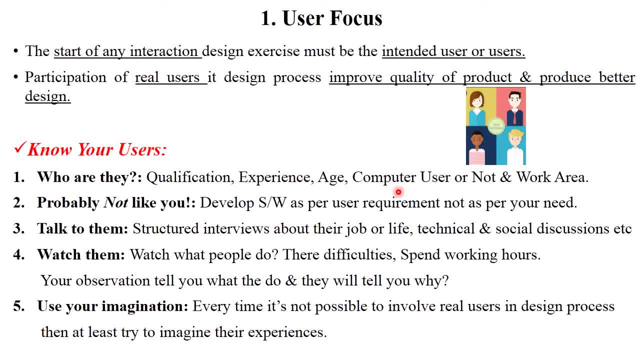 qualification, experience, age. your users are computer users or not. working area of users. you must know all those things before start the design or before start the development process. right, you must know each and everything about your customers. next: probably might not like. you means you should develop a software as per the user requirements, not as per your need. talk to them. 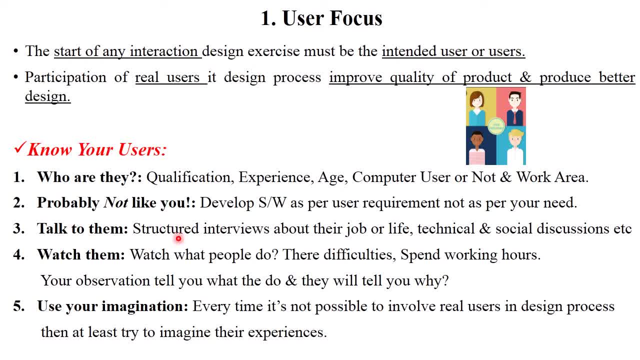 means you should Take a structured interview about their job or life. Some are technical and social discussion with your customers or with the users, So it's easy to understand what exactly user want or what exactly customers want. right, The next watch them. 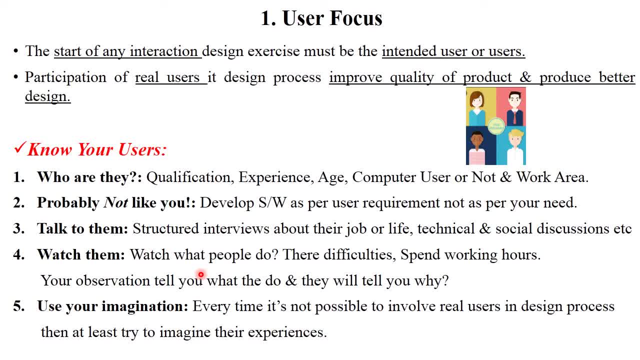 Watch what people do, what your customers do in their free time, in their working hours, what difficulties they faced, right So your observation tell you what to do and will tell you why. Right So you must know all those things regarding your customers. 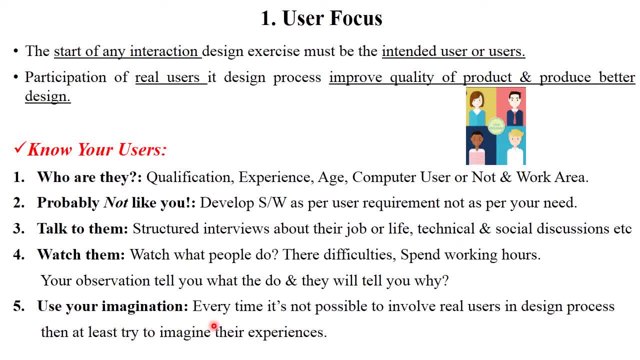 Next, use your imagination. So every time it is not possible to involve real users in design process, So at least try to imagine their experiences Means just imagine what the customers want and, as per the requirement, you should make a particular software. 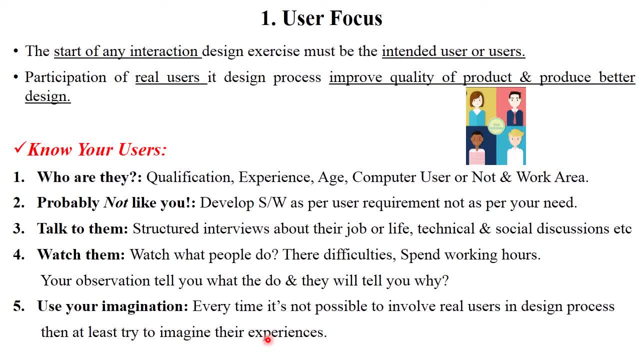 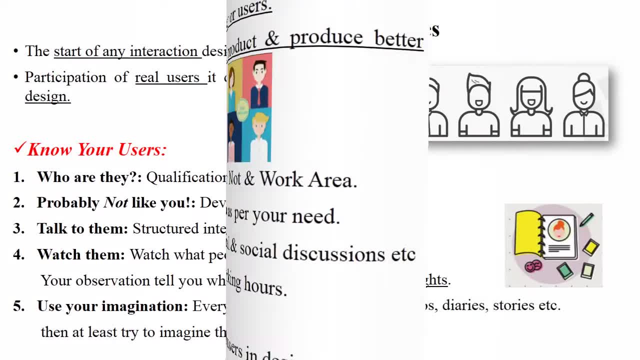 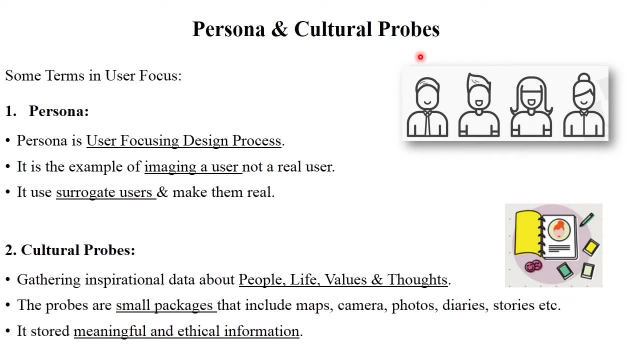 Right. So this all things is one of the most important or key part while designing software or development process, Right Next. The next is persona and cultural props. So these are the some terms regarding user focus. So persona means persona is a user focus in design process. 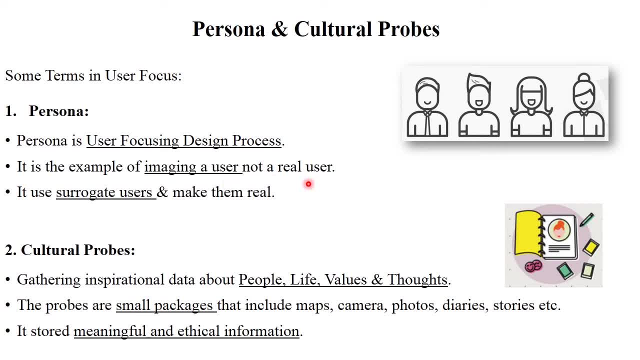 It is the example of imagine users, not a real users. Sometimes it is not possible to involve real users or real customers in development process or in design process Because there are some security issues, Right Right. So you should have a security approach in that. 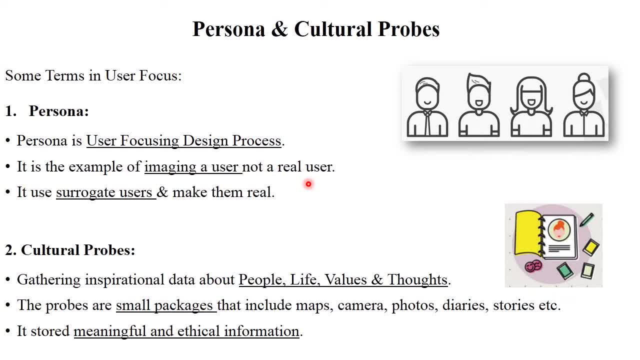 Right So at that time, just imagine what user want, what difficulties they are faced. Right So imagine at that time. So this users is called as surrogate users or not a real users, imaginary users. Right So, by thinking about that users and make them real, 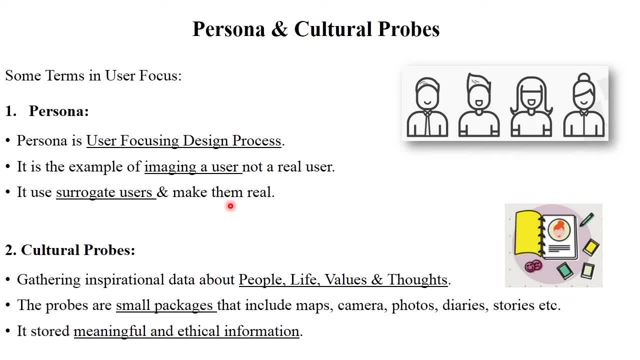 Fulfil each and every requirements or fulfill each and every difficulties they faced by developing a particular software Right that will be helpful to each and every customers in their working areas, right so this concept, by imaging a user, not a real user. this concept is called as: 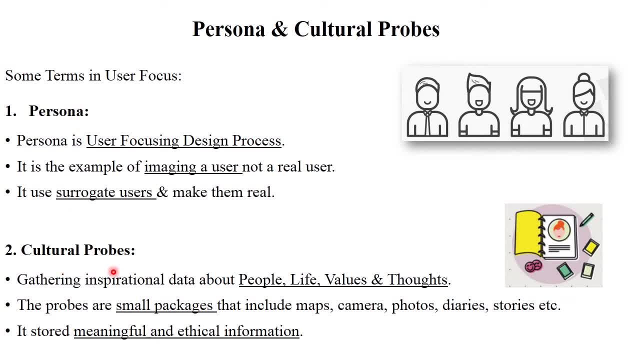 persona clear. next one is cultural props. cultural props simply means to gathering an inspirational data about people, life, values and thoughts, etc. see, the most real life example of cultural props is our social apps. by using social apps like whatsapp, Facebook, Instagram, then YouTube, by using this, we will cover our 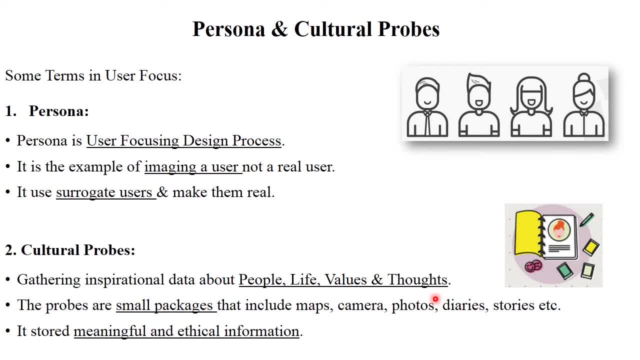 tych, ok, chatting functionalities, calling, then other, some payment applications- right, this, all kinds of functionalities are there, so it's easy to each and every users. there are some payments app like Google pay, paytm, so they fulfill their need, right, each and every users. okay, so this called as cultural props. the props are the small packages. 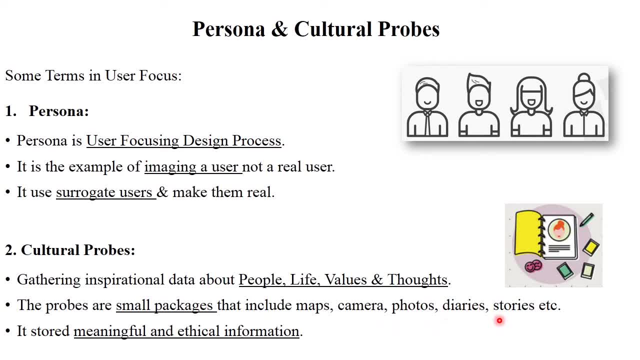 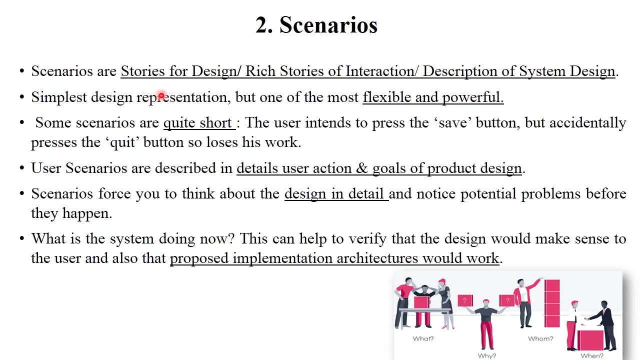 which includes maps, cameras, photos, diaries, stories, etc. so these are all the basic needs of each and every customers, right? so it store meaningful and ethical information. these things are called as cultural props, right next, the next and second uh, design constraint is scenarios. scenarios are story for design. reach stories of interaction and description of system design, when you should make 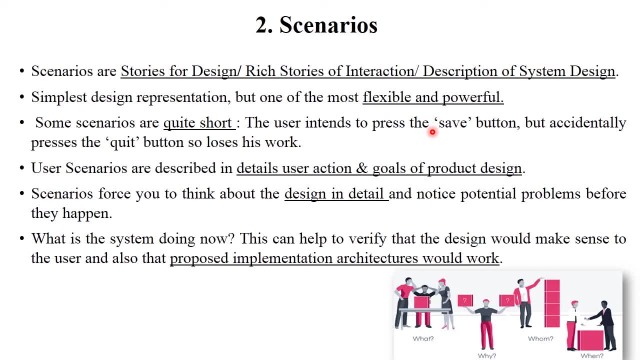 a particular design of that particular software. right so there are particular story behind that, right so this called a scenario: simplest design representation and one of the most flexible and powerful part. so scenarios are quick shot. like the user intended to press the save button but accidentally they press the click button so lose- they lose their work. this called as one scenario, right so there. 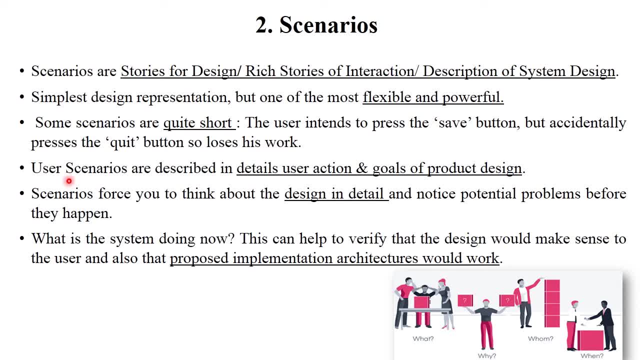 are different types of scenarios are involved in this process. user scenarios are described in detail in user actions and goals of particular product. design scenario force you to think about the design in detail and notice potential problem before they happen. okay, so scenario means in detail explanation about your design. what is the system doing now? this can help to verify that. 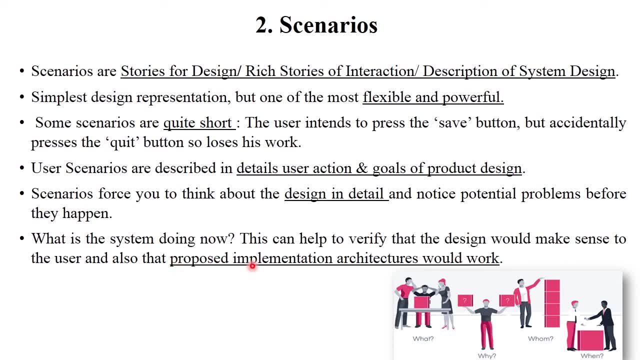 design would make sense to the users and also proposed implementation of architecture. and course not by using scenario. suppose in future there are some particular problems are generated, will be generated, so by using scenario you can solve those problems in before steps, right? so scenario means simple or description of your design, clear. next, 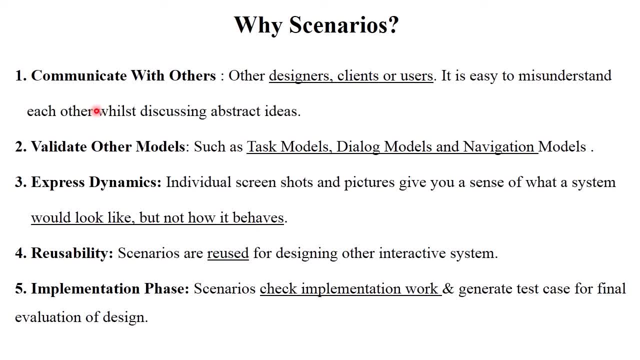 one is why scenarios communicate with others. you should communicate your designers, client, users, so it's easy to misunderstand each other while discussing abstract ideas. there is particular combination or communication between the designer, programmer, developer or the tester, so they make your product will be more intelligent. way right. so validate other models, such as task models, dialogue. 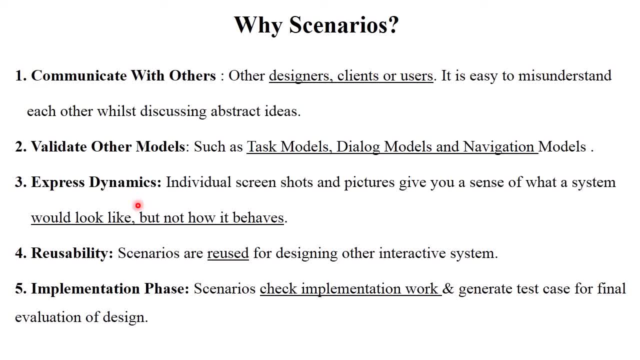 models and so on. navigation models express dynamics. it means individual screenshots and pictures give you sense what system would look like, right? so by using design, you must know that, what systems will look like, but not how it behaves. okay, so how it behaves, it's completely a implementation part. 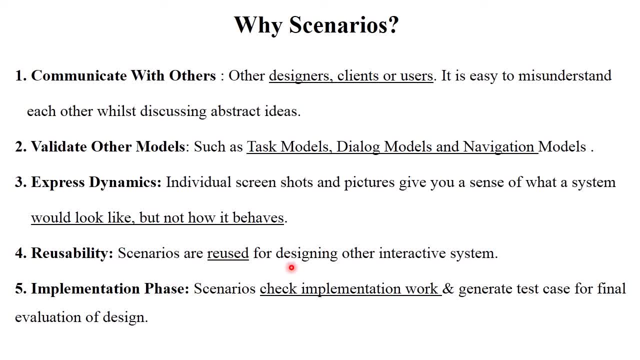 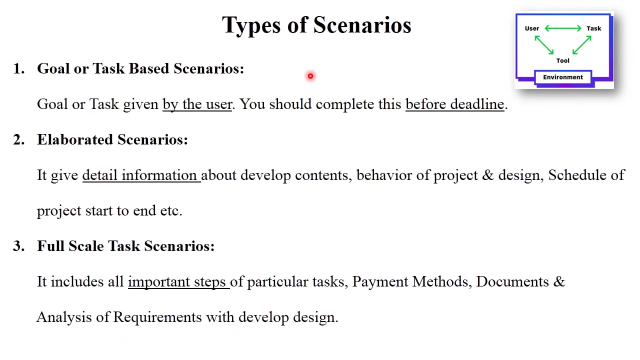 right. the next reusability scenarios are used for designing other interactive system right. then implementation phase scenarios: check implementation work and generate a test cases for final evaluation of design developer. design developer: develop a particular product by using the scenario of particular design right. next types of scenarios: there are four for three types of scenarios: goal or task. 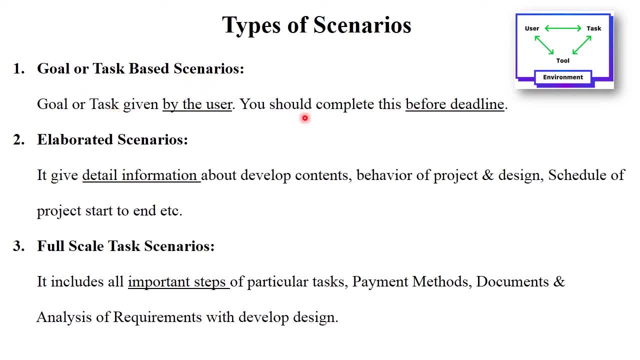 based scenarios. so goal are tasks given by the user. you should complete your project before the deadline. next, elaborated scenarios. elaborated scenarios means it gives the detailed information about develop contents, behavior of project, design and sharing of project, whether the particular project is start and end. so this all type of life span is called as elaborated. 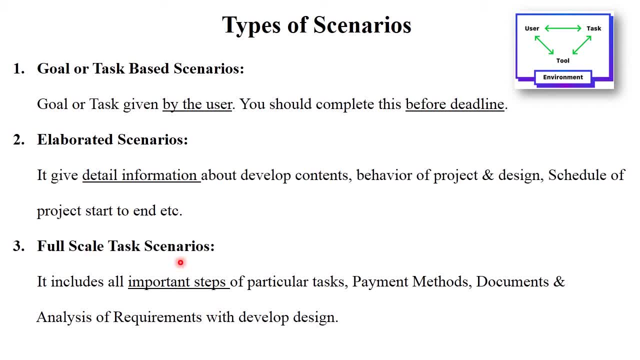 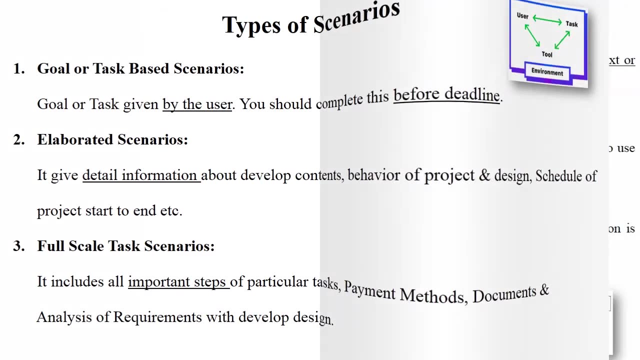 scenarios. the next one is full scale task scenarios. it includes all the important steps, like particular tasks. there are some payment methods, documentaries and analysis of requirements with develop design. so these are called as types of scenarios, right. Next, The third and important constraint is navigation design. So navigation is the process. 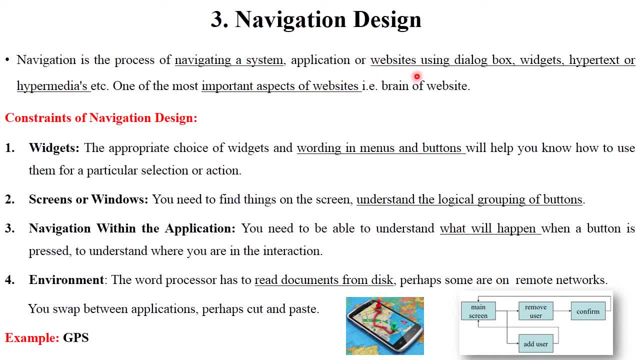 of navigating a system, applications or websites using a dialog box, widgets, hypertext or hyper medias, etc. So navigation is one of the important aspects of website, which is also called as brain of websites. right, Then you should click on particular link so it moves to another page. 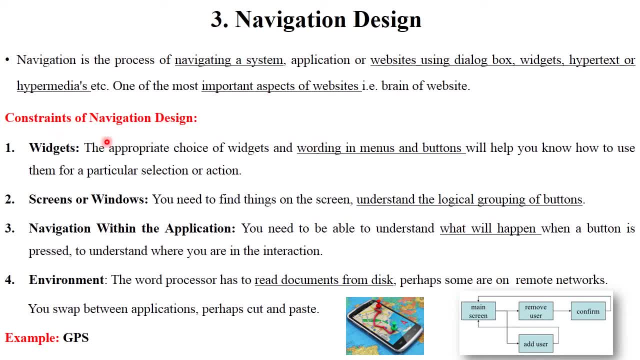 This is called as navigation. There are some constraints of navigation design. First is widgets. The appropriate child's choice of widgets and writing in menus and buttons will help you to know how to use them in a particular selection or action. You must know whether you should use. 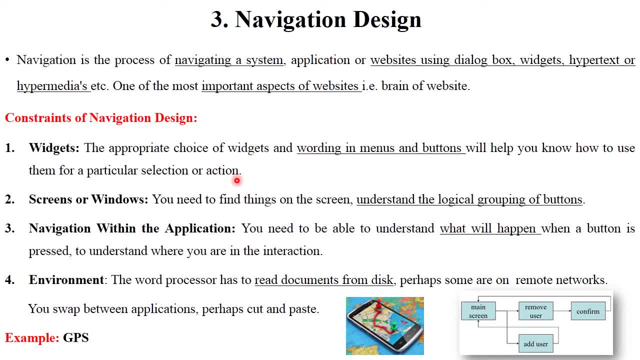 button, whether you used checkbox, radio buttons in your design, right, You must know all those things. Next screen or windows. You need to find things which are not in your design. So you need to find things which are not in your design. 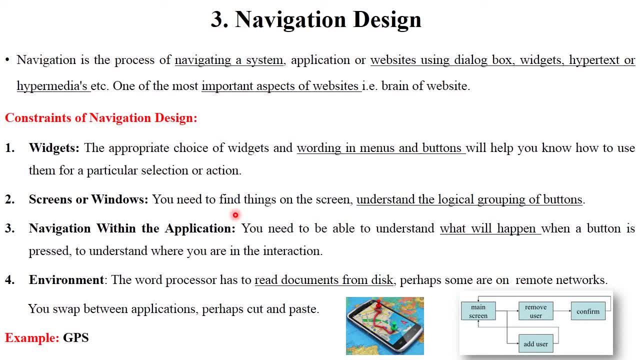 Which things or which types of buttons applications are present on the screen. It understand the logical grouping of button right, Next navigation within the application. You need to able to understand what will happen when button is pressed to understand where you are in the 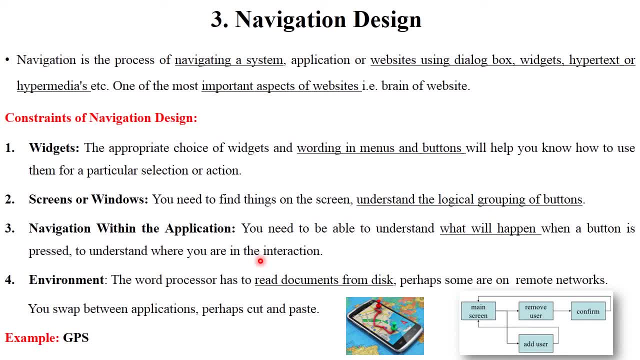 interaction. You must know the action of each and everything: Environment- Environment means the word processor has to read the documents from disk. Perhaps some of the remote networks swap between application, cut paste. These all things are included in your environment, right? 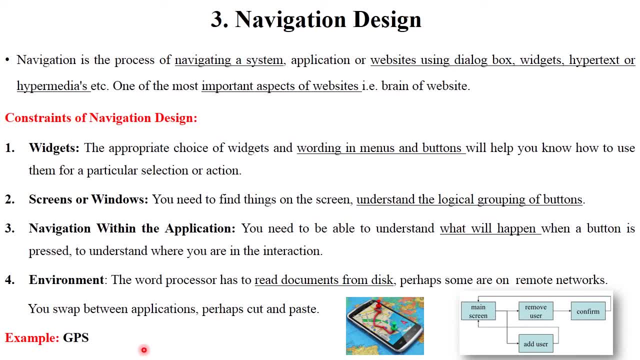 The best example of navigation design is GPS system. GPS shows source to destination: shortest path right. It shows the pointers from left direction, right direction. If there is traffic is present on the road, it shows in red color right, Or it also shows whether you are located. 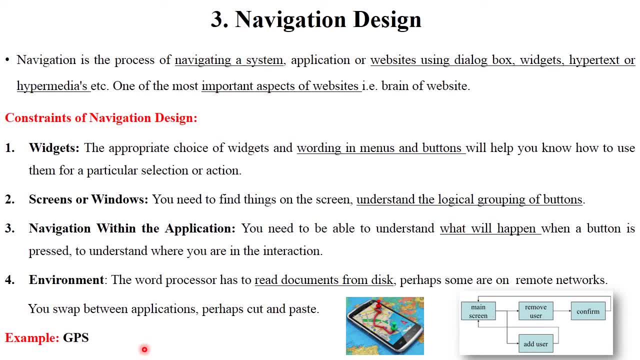 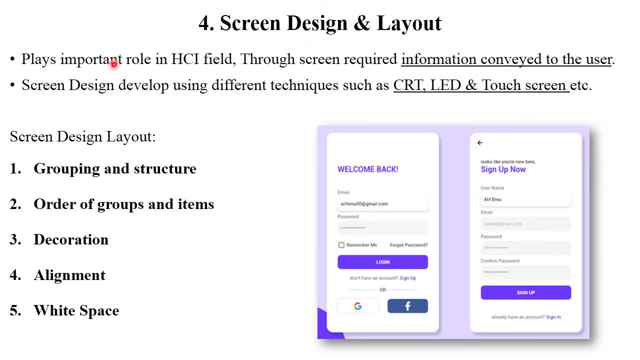 So these are the important navigation. So you need to know all those things. You must know the navigation of GPS system right Next. the next and last constraint is screen design and layout. Screen design and layout plays the important role in human computer. 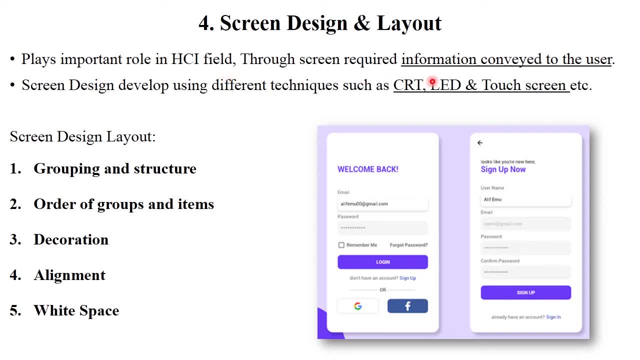 interaction field Through screen is required information conveyed to the user. Screen design developed using different techniques like CRT, LED, touch screen, etc. Right So screen design is one of the most attractive part If you design your software. what is the most? 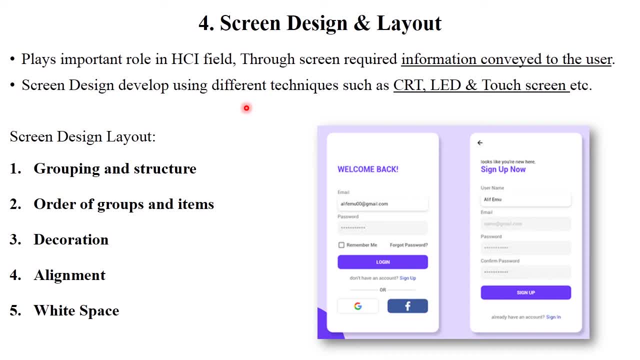 attractive way or informative way, So it's very good product or quality product, right. So screen design layouts includes grouping and structure, order of groups and items, decoration, alignment and white space- right. See here. this is just example of screen design. 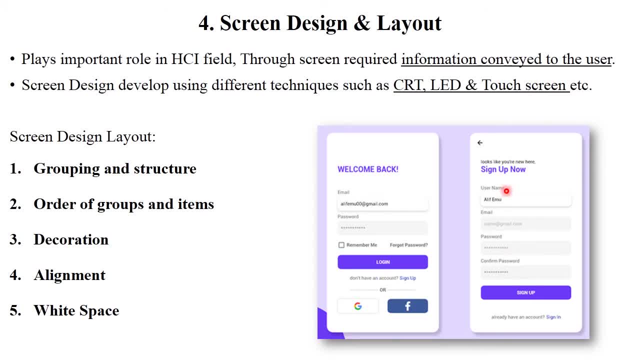 the login page and sign up page. Wonderfully, these all things are designed and only required information are stored right. So this is the best example of screen design and layout. So screen design is one of the most attractive way or informative way. So screen design. 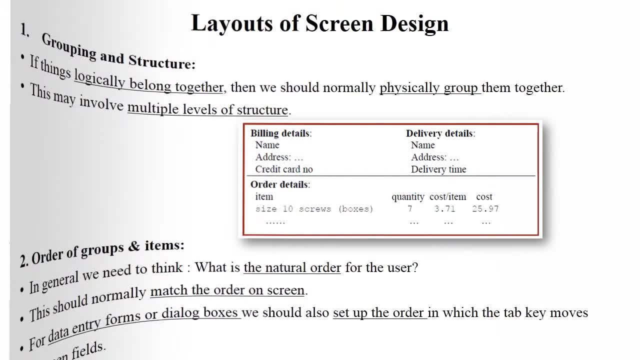 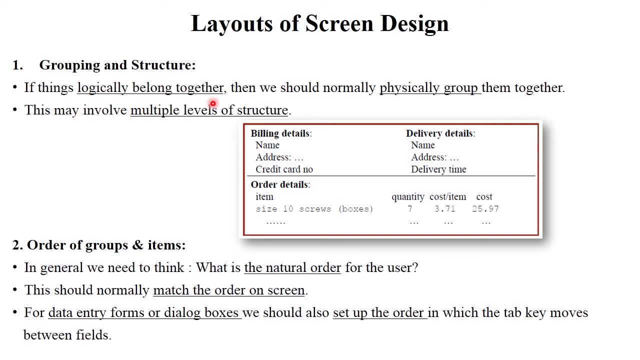 is one of the most attractive way or informative way. So screen design layouts includes grouping design, next lots of screen design in detail. the first is grouping and structure. if things logically belong together, then we should normally physically group together, right? so this may involves multiple levels of structure, and another is order of groups and items in general. we need 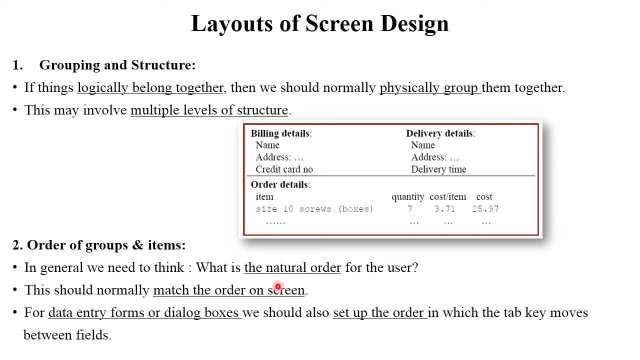 to think what is the natural order of the particular user? so this should normally match the order on screen. see here. this is just example of grouping and order. the first one is billing details. so billing details means these are the one group, like the name, address, credit card number etc. 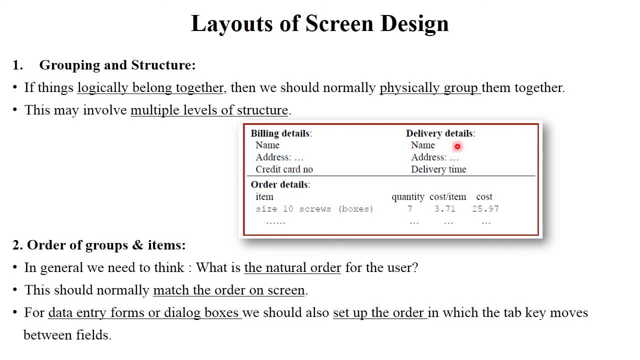 means: group together, okay, delivery details. delivery details also includes name, address, delivery time. right then. order details means: suppose particular item, their quantity is 7, their cost, etc. right, so, group together as per their order. this is the particular layout of this particular design. right, so this is. 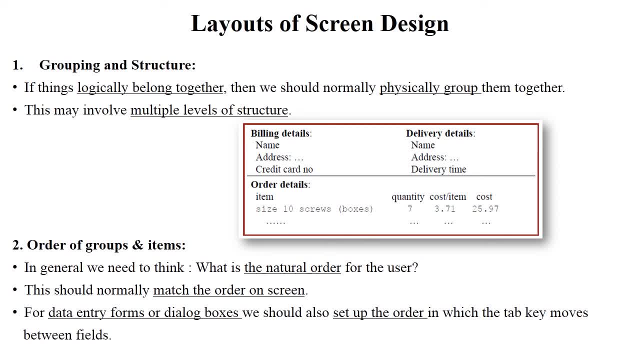 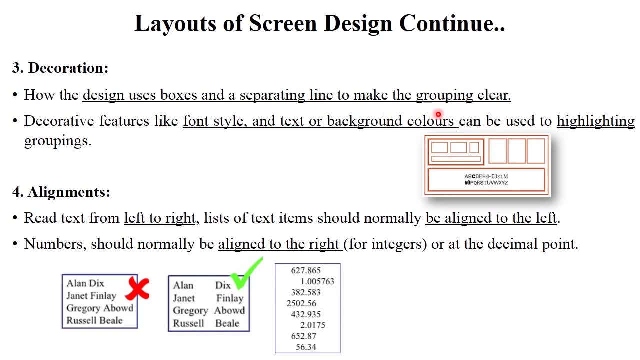 the sorted structure clear next. the next is decoration: how design use boxes and separating line to make the grouping clear. decorative features like font style, text, background colors can be used to highlighting the groupings. so this is one of the most attractive part. that is decoration. you should make a particular 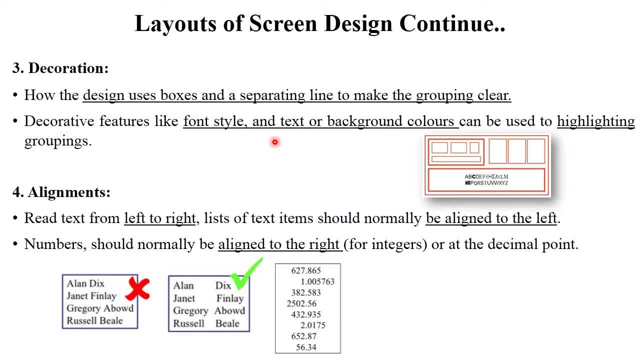 software by appropriate designing, by sorted manner, etc. right. the next one is alignment. read text from left to right. list of text item should be normally be aligned to the left. number should be normally aligned to the right part or the decimal part, see here align disk. so the first. 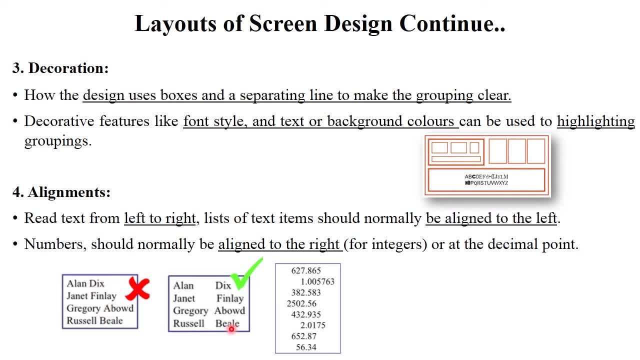 name and last name are not properly arranged, but in this way the first name and last name, last name, are properly arranged in tabular order format. right, so this is the most effective way. now, see here, this is decimal part, like 2.27.86, so decimal parts are properly arranged in this way. okay, so while making a design of particular, 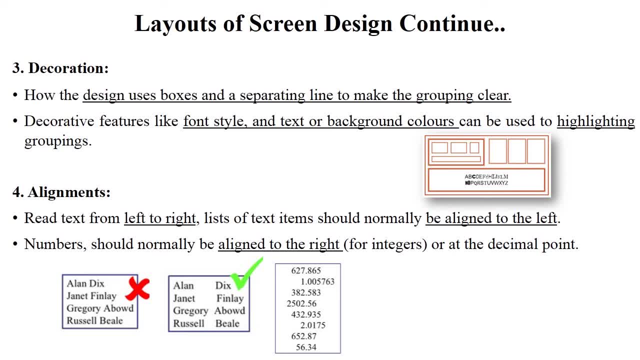 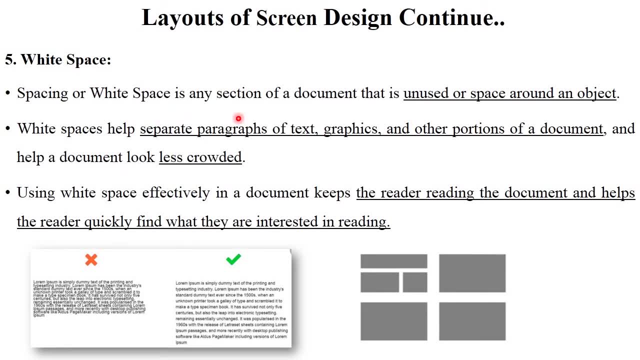 software. you must remind these things, decoration and alignments, clear. next, the next and last is white space. so spacing or white space in any section or document that unused, or space around the object right. So white space helps the separate paragraphs of text, graphics and other. 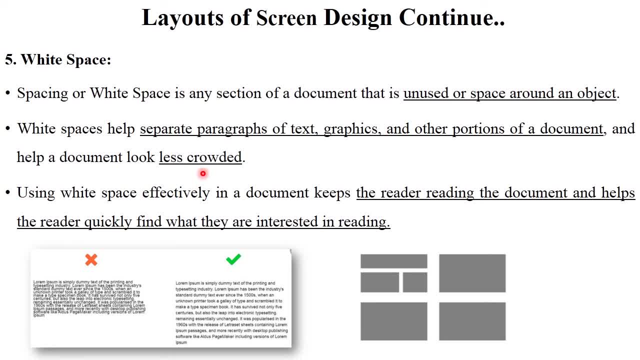 portions of documents. It helps a document look less crowded, right. So using white space effectively in document the reader reading the documents and help the reader quickly find what they are interested in reading. alright, See here. So this paragraph is not as much attractive. 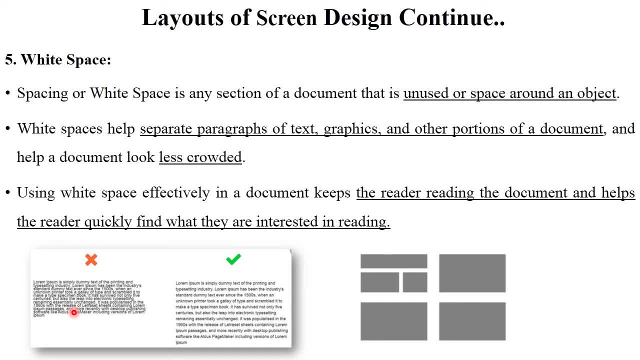 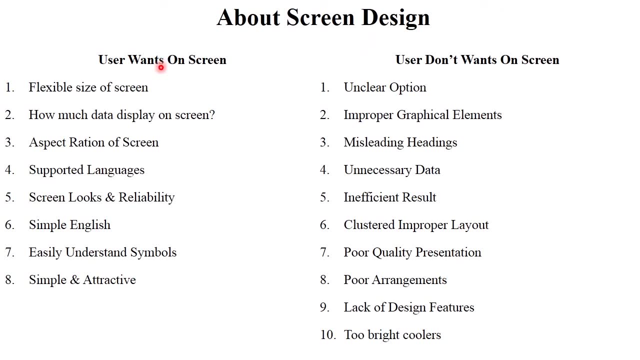 but by adding appropriate white space. this must be attractive, easy to read, right. So this is the white space is one of the most important while designing a particular product. Clear Next. Next about screen and design: What user wants on screen? User wants flexible. 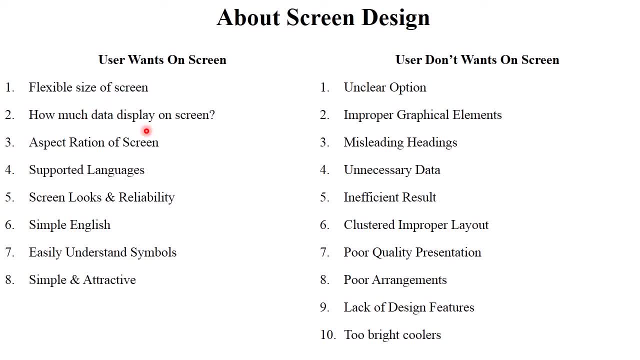 size of screen right. How much data display on screen. Aspect ratio of screen. Supported language like English, Hindi, Marathi, English Hindi, Hindi, Hindi, Hindi, Hindi Hindi Hindi. there are various supported language for the keyboard. Then screen looks and reliability. 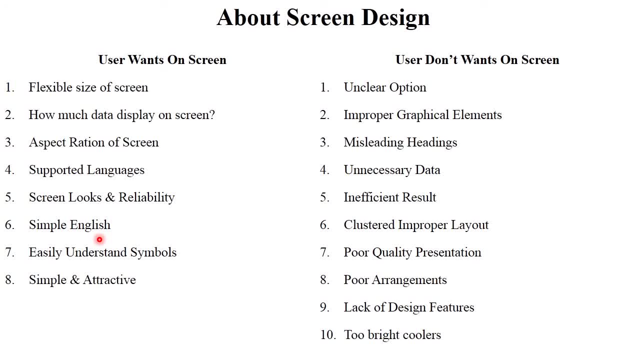 simple English language So it will be used for each and every person easily understand symbols, simple and attractive. So user wants all those things on screen. But what user don't want? Unclear option, improper graphical elements, misleading heading, unnecessary. 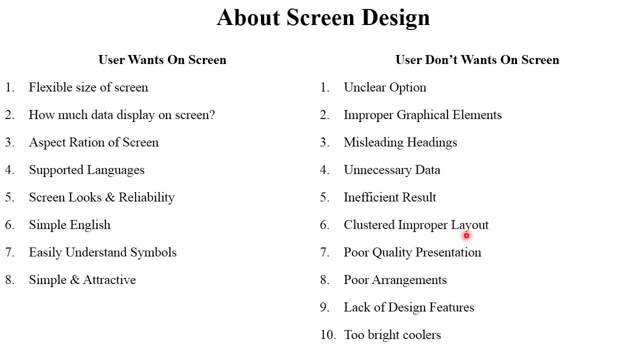 data inefficient. result: clustered improper layout, then poor quality presentation, poor arrangements, lack of design features and too bright color. These all things user don't want on screen. okay, So while designing or develop a particular product, you must remind those things what your customer want or what they don't want on particular screen.